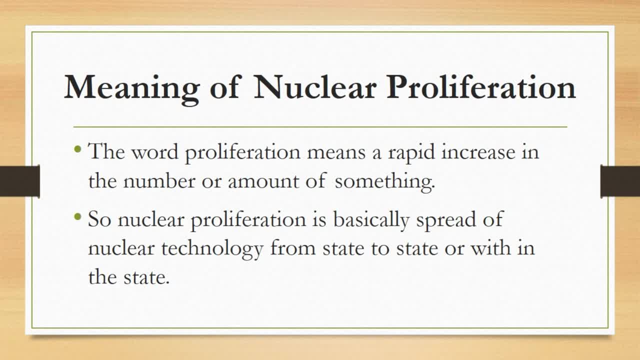 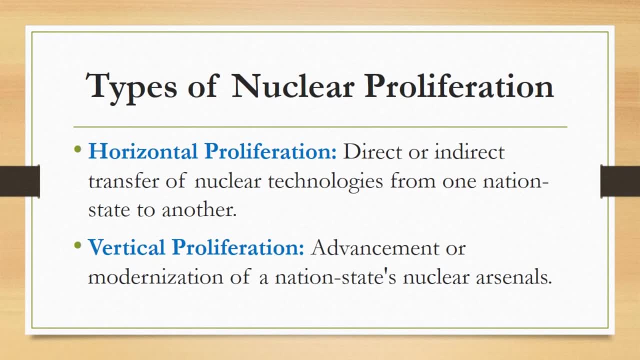 proliferation is basically spread of nuclear technology from state to state or within the state. Now, what are the types of nuclear proliferation? There are two types of nuclear proliferation. One is horizontal proliferation and other one is vertical proliferation. Horizontal proliferation is the direct or indirect transfer of nuclear technologies from one nation state. 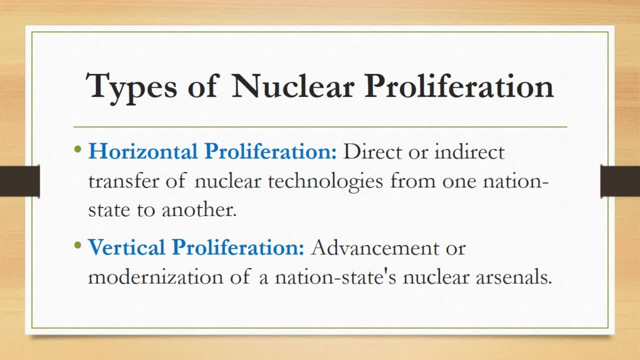 to another, Whereas vertical proliferation can be defined as the advancement or modernization of a nation state's nuclear arsenal, Which ultimately leads to the advancement of developing a nuclear weapon. From these two types of nuclear proliferation we can make a concept that if the number of the states 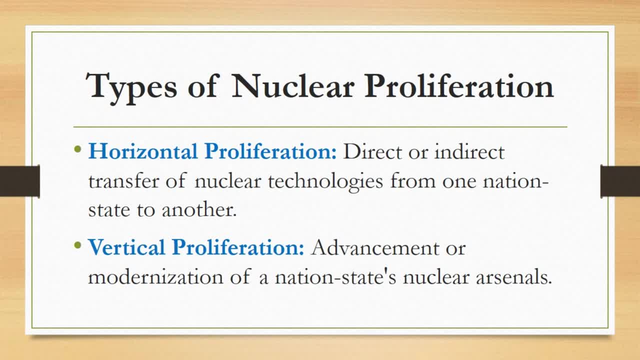 possessing the nuclear technology increases, then we will say that horizontal nuclear proliferation is taken place. And if the nuclear technology of a nation already having this technology increases either quality or quantity of its nuclear weapons, then horizontal nuclear proliferation is taken place. History of Nuclear Proliferation. 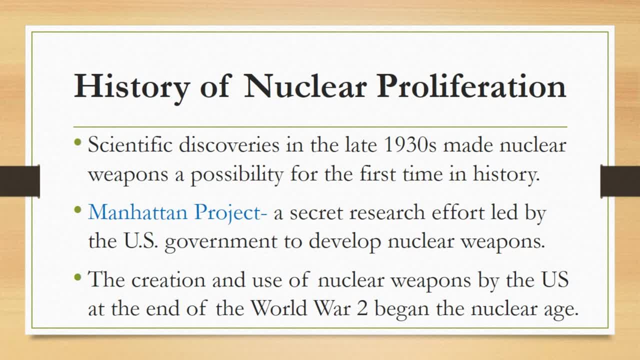 Scientific discoveries in the late 1930s made nuclear weapons a possibility for the first time in history. During World War II, the United States and its allies were afraid that their enemies would develop nuclear weapons First. so in 1942, they started the Manhattan Project, which was a secret research effort. 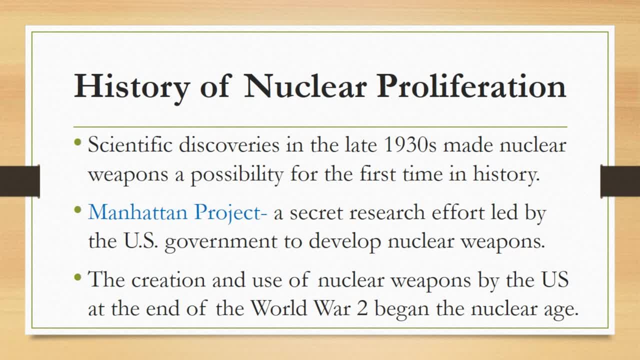 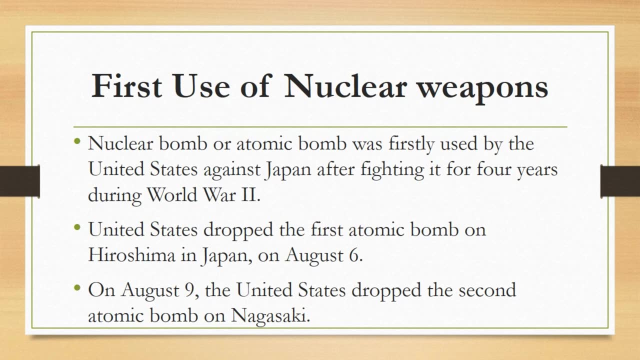 led by the US government to develop nuclear weapons. The creation and use of nuclear weapons by the US at the end of World War II began the nuclear age- First Use of Nuclear Weapons. Nuclear bomb or atomic bomb was firstly used by the United States against Japan after fighting. 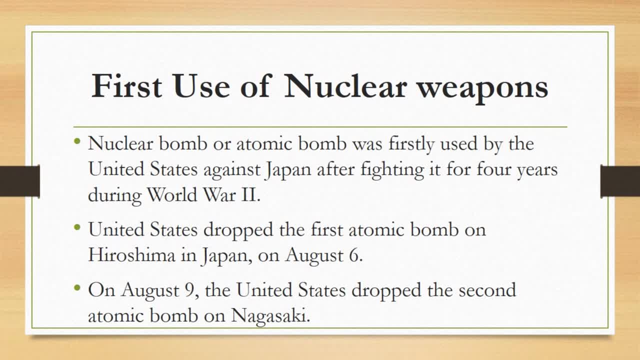 it for four years. During World War II, the United States dropped the first atomic bomb on Hiroshima in Japan on August 6.. This attack killed more than 100,000 people. On August 9,, the United States dropped the second atomic bomb on Nagasaki, which killed more than 70,000 people. 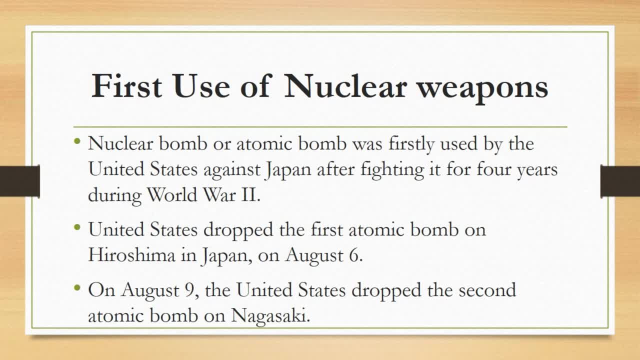 Six days later, Japan announced his country's surrender. Those atomic bombs remain the only ones that have been used against the United States. Second, Use of Nuclear Weapons. Nuclear Weapons: Nuclear Weapons ever used in war, because since then few countries could achieve this technology but cannot use it. this attack by the us put world in the new race, this race. 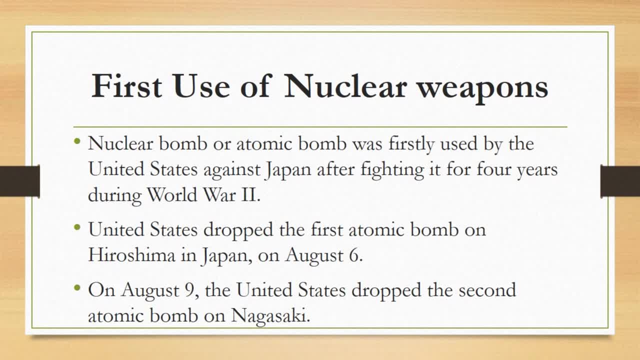 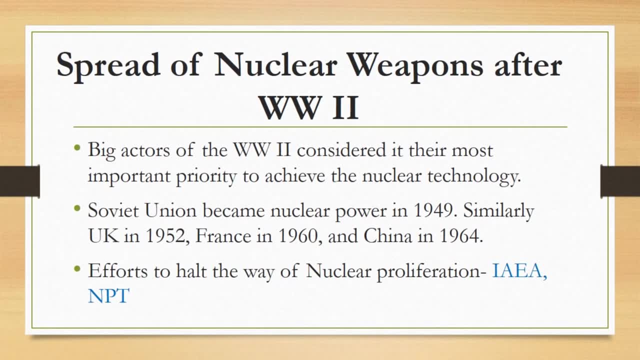 was to achieve the nuclear technology. as a result, the nuclear proliferation got pace in the world after World War two. spread of nuclear weapons after World War two. the drastic end of World War two was the beginning of a drastic race of achieving the nuclear technology. big actors of the World War two considered: 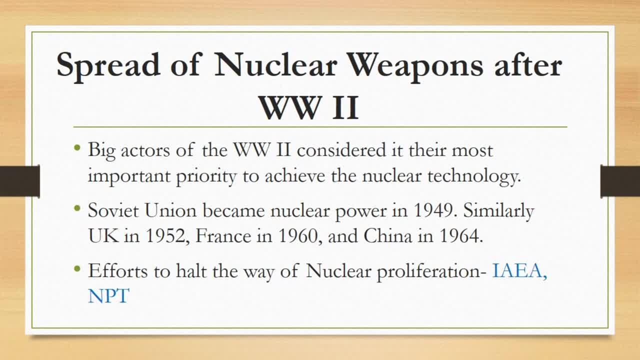 it their most important priority to achieve the nuclear technology. as nuclear technology had emerged as the most powerful and decisive technology at that time, countries started fast research in this regard and opened the avenue to the world war two. just four years of first use of nuclear weapons by the United States, the 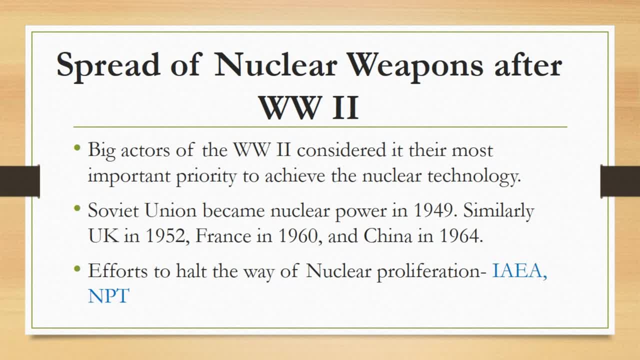 Soviet Union conducted its first nuclear test explosion in 1949. similarly, the United Kingdom got nuclear power in 1952, France in 1960 and China in 1964. in few years there were five nuclear weapons states in the world. this pace of horizontal nuclear 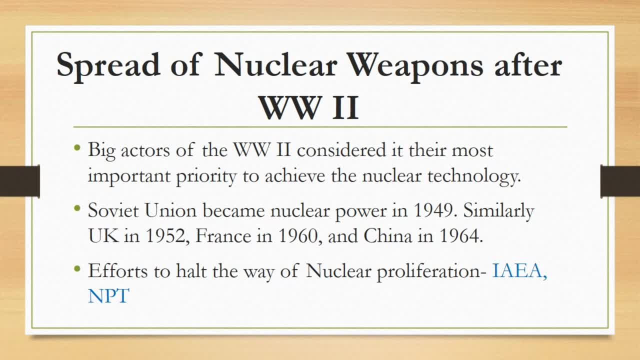 proliferation became a new threat for the big parts. they were worried that if this process would not be stopped then the whole world may got this technology and world would be blown up at any time. as world had witnessed the damages caused by the first use of nuclear weapons by the United States, some steps taken. 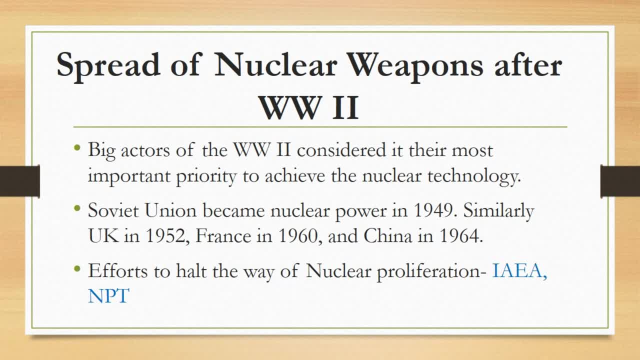 immediately to stop this race. the establishment of international atomic energy agency, that is IAEA, and the signing of nuclear non-proliferation treaty, that is NPT, played their important role to stop this proliferation. but still India and Pakistan succeeded in achieving this technology in 1998 because they were not 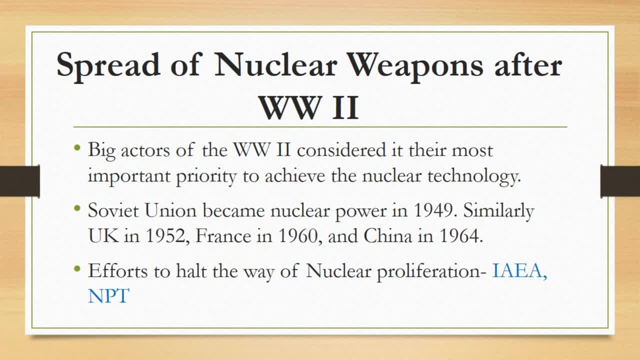 signatories of NPT nuclear non-proliferation treaty has been covered in detail in another lecture, the link of which is available in description. so this was all from today's lecture. thanks for watching this video and I will see you in the next one.